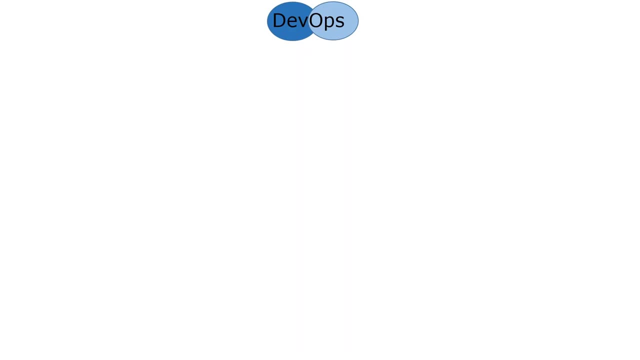 new topics or concepts. That is W2H principle. If you can see on the right side top, that's W2H principle. So what is the W2H principle? So two W's and one H. So two W's are what and why and one H is for how. So what is the 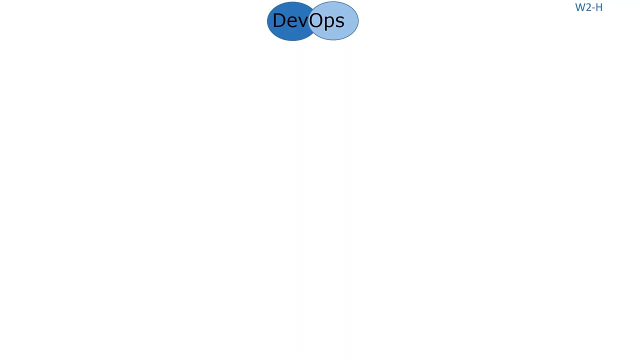 concept all about. Why are we using this concept And how are we going to implement this concept? So this practice makes you more and more comfortable to understand any particular new topic. So let's get started. Let's get started. Let's get started. 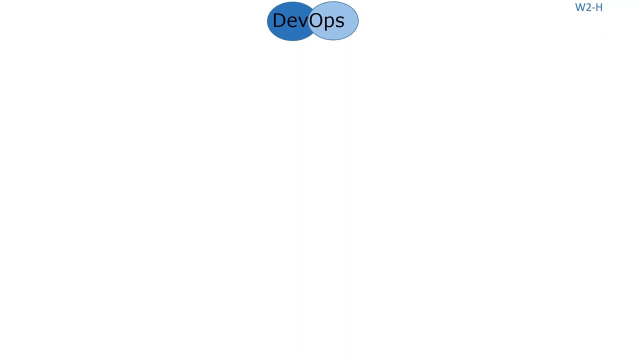 Now let's get started. DevOps is a concept or content, So please do follow, if you like, this principle. Okay, let's jump to the topic now. So what is DevOps Culture? to streamline the release process, improving product offerings with better team. 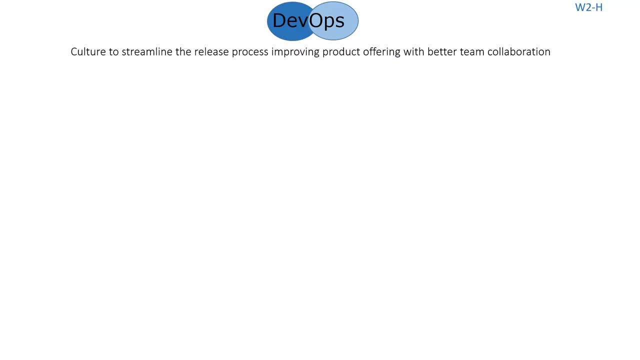 collaboration. What does it mean actually? A DevOps is a culture or set of practices or a mindset which tries to enable the team to collaborate or combine or form a transition Form, a transparent layer to bridge among the teams so that each and every member in the team 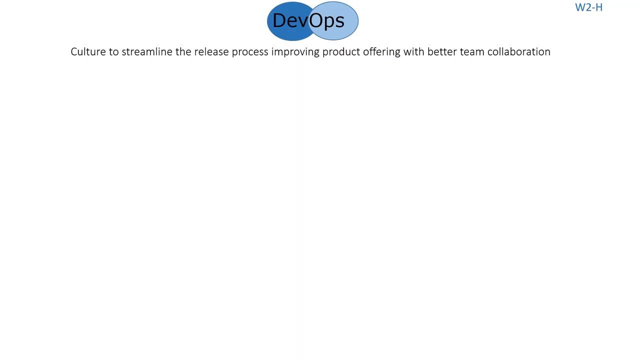 Gets involved and solve each other's problems, So working together for speed and stability. Before implementing devops, We should be aware of the team's development model, SDLC, That is, software development life cycle. Let me explain you that first. So software development life cycle, HDLC, is a methodology, how the teams in the organization are. 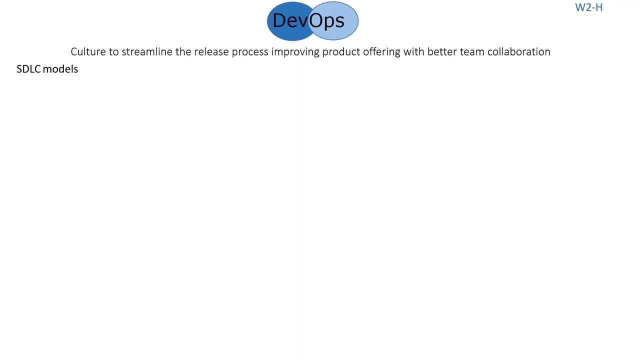 Designing the development work into multiple phases to improve the design product and product project management. So there are multiple models for SDLC. in this video I am going to explain you few of them. Let's go. Yeah, there comes. and this is one of the old SDLC models called waterfall model, where project activities like requirement 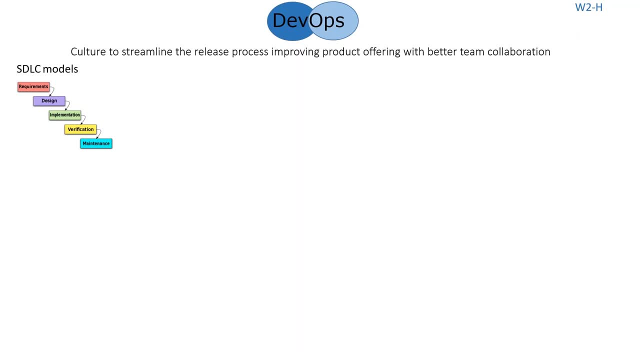 design, implement, verification and maintenance are. break it down into linear, sequential phases where each phase depends on the deliverables of the previous one, Means it is like less iterative and less flexible approach, because the progress flow goes from our one direction downwards like a waterfall Which lags in revisiting or revising any prior phase once it is completed. 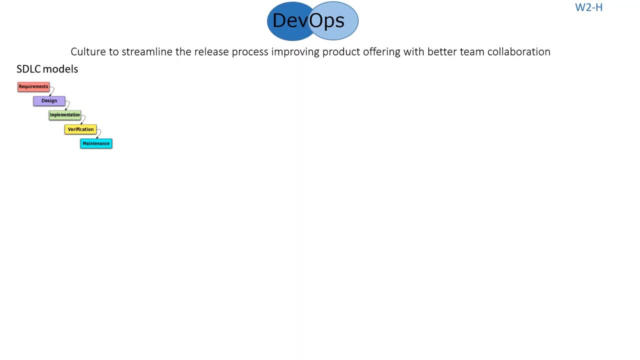 So, which is one of the drawbacks of waterfall model, and of course, it takes a longer delivery time. and Next comes is a V model. So, if you can see in the picture, V model is to tends to be our extension to Waterfall model, instead of moving downwards in a linear way. 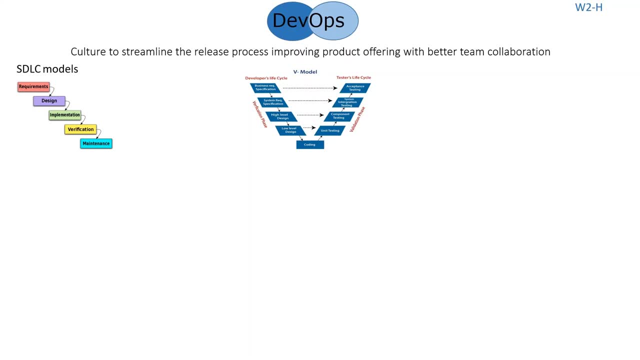 It is bent up towards the coding phase to form our V shape, Where left side of the V Is our verification phase and the right side is a validation phase, if you can see there, so what happens? So this makes tough to get the software design in the early stages. 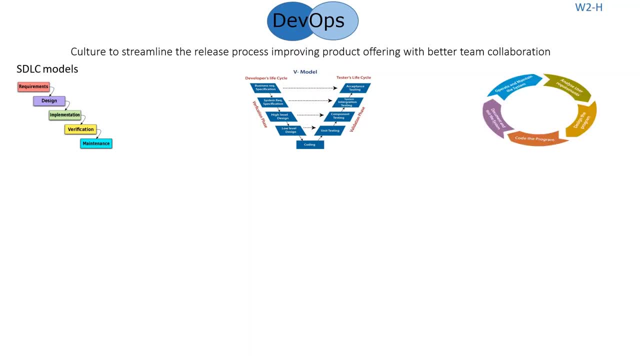 Okay. So on the other hand, we have a agile, which is the latest software development models. So it is a iterative development model where teams are mature enough to pick the requirements, break them into pieces, discuss and individual members of the team Given the importance and flexibility to choose. the task is good with. 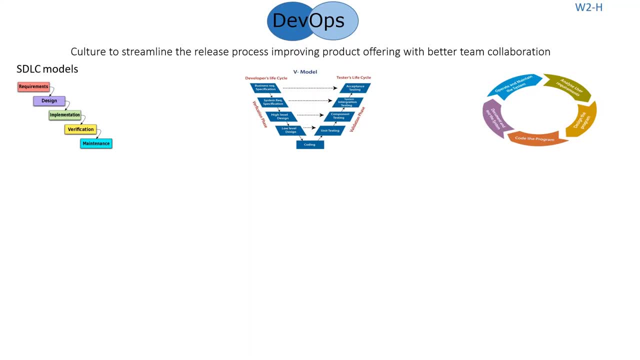 Release of the product is done as a smaller pieces, With short business benefits in the early stage of development. everyday interactions with a team develops better communication. So this is how the three HDLC models are been designed and Moving forward. now let's discuss on DevOps. 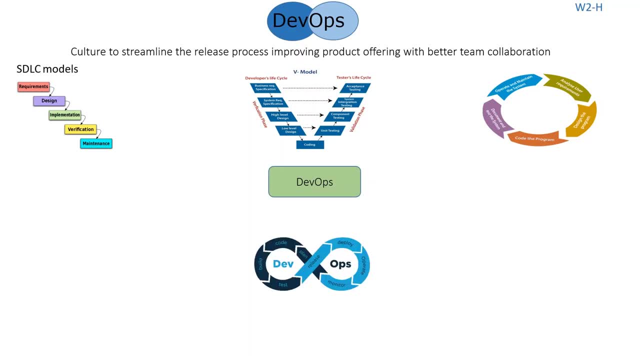 So if you ever discuss about DevOps, there will be a buzz Like: there will be involvement of development and operations. and what are these teams? so two teams are mainly involved. one is a development team, other one is the operations team. so let's talk about development teams, which is dev. so dev is a shorthand for developers in particular. 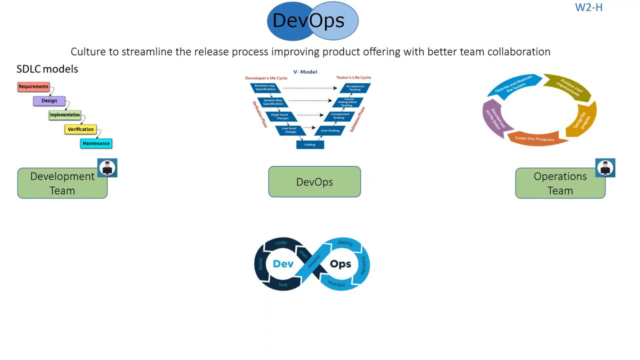 but really in practice it is even wider and means all the people involved in developing the product, which can include product QA and other kinds of principles. so this will bring the teams closer and eliminates a gap between them. that means the testing team and development team work together- the dev and whereas the 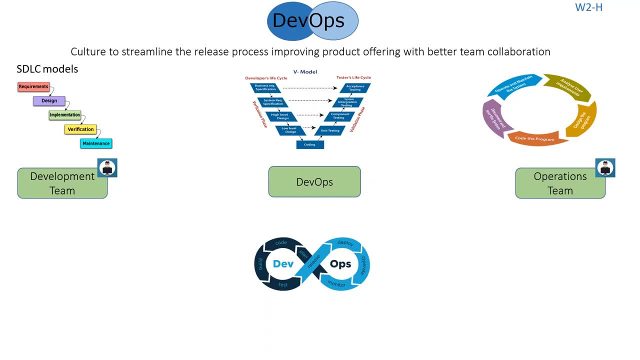 operations team. operations team is a combination of system engineers, system administrators, operation staff, release engineers, DBS, network engineers, security professionals. they are responsible for development, maintenance, monitor and fix the errors. so this idea on development team and operations team. now let's see how the bridge has been formed between the two teams. so moving to next is the 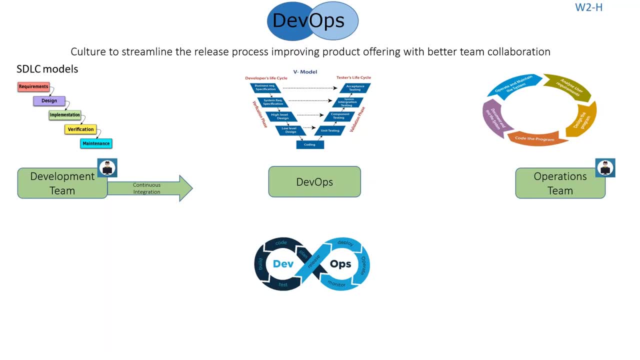 continuous integration. so what is continuous integration? so it is a practice of merging and testing the code every time developer pushes the changes into a centralized source code manager. this is the best practice to avoid conflicts and helps to detect the problems in the early stage of development by validating the software as soon as it is pushed into the source. 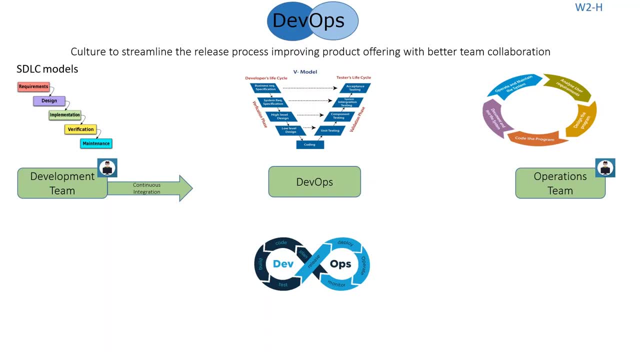 control system and next, it is a continuous delivery. so continuous delivery, what is this? this process helps to deliver the software updates to release in a smaller increments, ensuring that software can be released at any time, in other words, we can say it as a state of of being ready to release. this will lead to faster releases and, from the 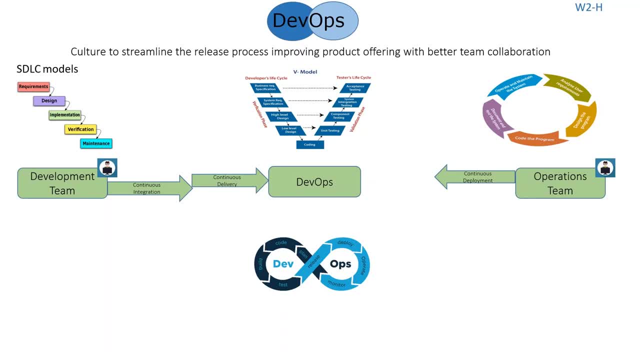 operation side we have continuous deployments, so the ability to deploy automatically to the production continually and give the feedback of the deployment process. and next one is a continuous monitoring. continuous monitoring refers to the process of implementing some monitoring across the each phase of software development lifecycle. this continually ensures that 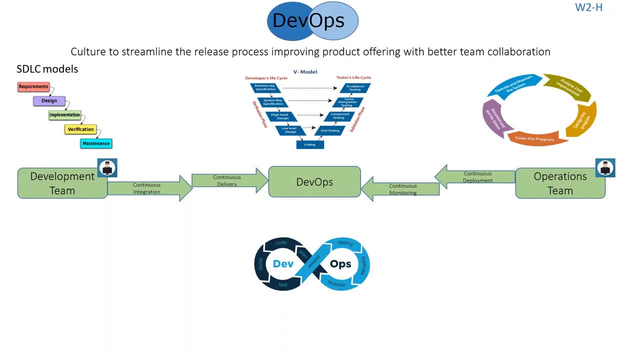 the health, performance and reliability of the software, upgrading from development environment to the production one. so these about the teams and how the bridge is being filled with the DevOps principles. now let us talk about the five core principles of DevOps. so if you see, there are five core. 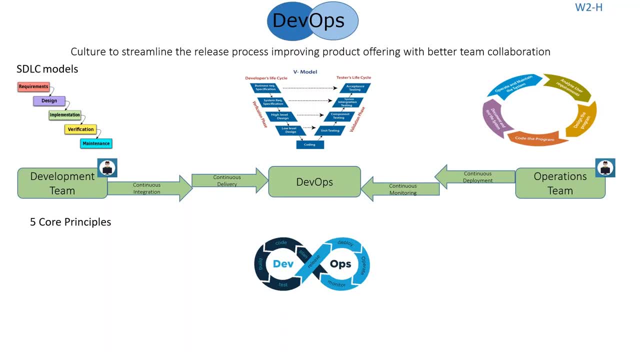 principles about the development and security process and also five core of DevOps. so the first one is the culture. so what is the culture? so culture is something shared responsibilities for developer development in deployment and operations. so sharing discoveries, practices, tools and learning across silos is increased on this culture. and next comes the automation. automation is 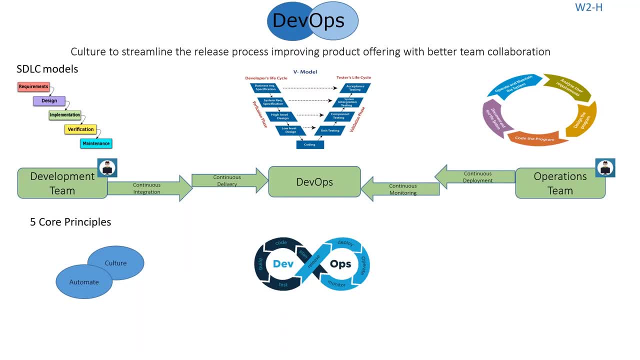 a key for DevOps to avoid manual, reusable stuff, automate the lifecycle using a continuous delivery pipeline, building the tool chains to help teams and focus on automating healthy process. and next comes is the lean. lean is to maintain smaller batch sizes, limiting the work in progress and extreme 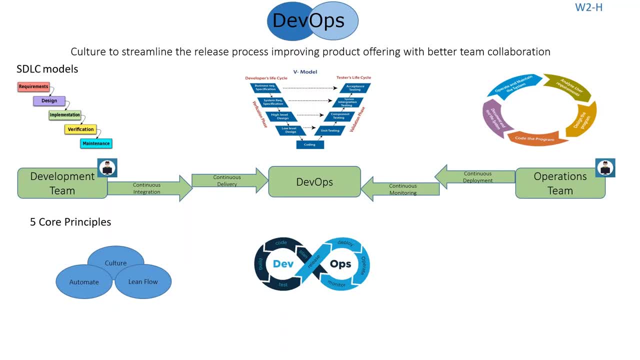 visibility. it accelerates the delivery by reducing the key lengths. so if there is a task, we always try to avoid doing a lengthy task and we concentrate on MVP- minimum viable product. so next comes is the measurement. so measurement is a very key for any process, not only for DevOps. any process, so measurement is like. 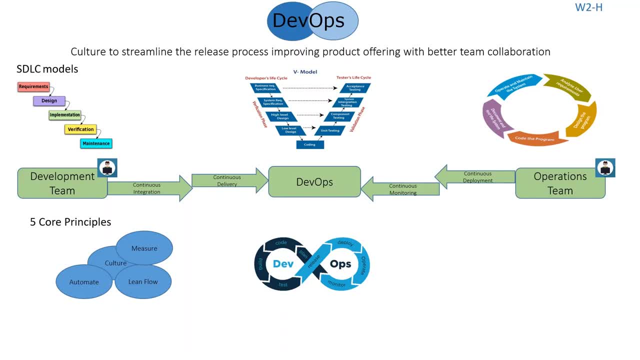 measuring the flow of development, development through pipeline telemetry, broadcast the measurement and continuously try to improve the measurement or the telemetry before and after problem solving. now the final one is a recovery. so what is recovery? so having our, you are already aware of that one. the recovery means something with the 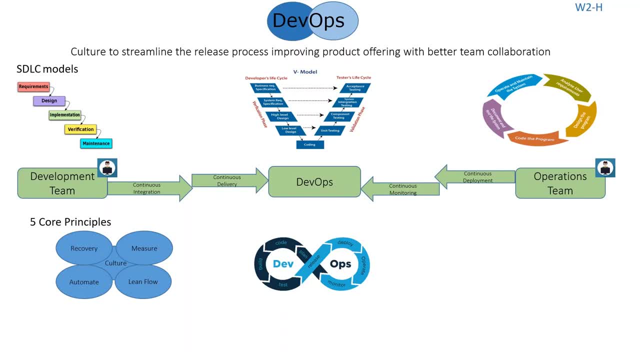 enabling low risk and forced recovery model architecture for fast reversion and fast fix over. Plan for failure: rehearse like chaos monkey. so what is chaos monkey? plan for failure: rehearse like chaos monkey. what is chaos monkey, pre recovery? first, this is the previous democracy: long-term it is seen and focused. 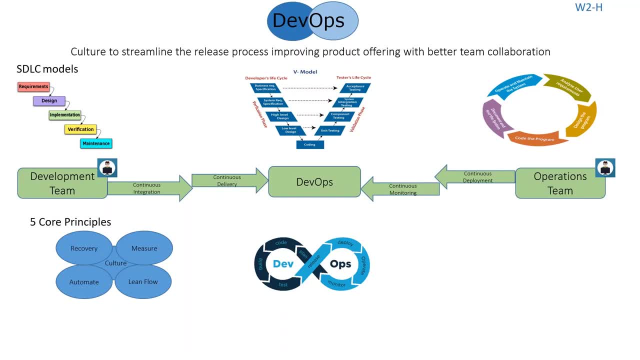 what is chaos monkey? chaos monkey is a tool designed by netflix to test the resilience of the it infrastructure through inducing specific type of failures, randomly shutting down the instances in order to simulate random server failure. so altogether it's a again on new topic and i'm going to explain you on the next video. so these are the five core principles and every. 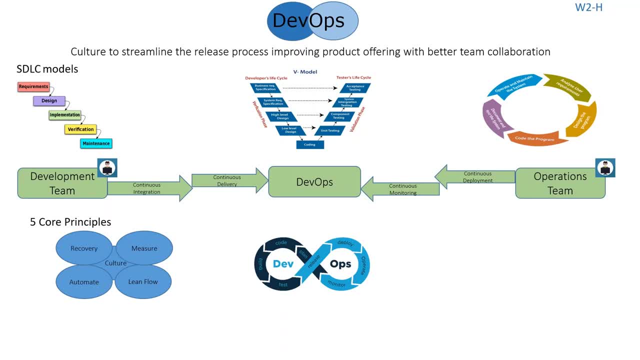 team should adapt this five core principles to be a successful devops team. now let's talk about the benefits. so what are the benefits devops provides? so if you see the first one, the foster lead time means what is the lead time actually? the time elapsed between the order and the delivery. 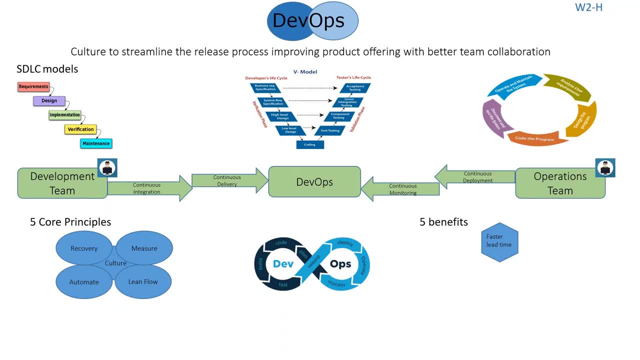 so by using devops you can experience the 440 times increase in the lead time means the lead time, the time elapsed between order and the delivery. you will get faster by using the delivery pipelines and fewer defects. we use lot of tools to scan the product before it goes to deployment so that the errors or the defects can be decreased by 96 times. 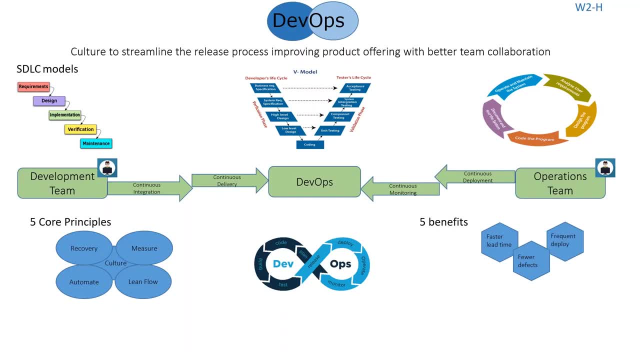 and next comes is the frequent deployments. so how frequent we can do the deployments by using devops. so we use pipelines, so frequent deployments can be done over 46 times to shorter pipelines and more delivery cycles. so next comes is the faster recovery as a product is passed through the same. 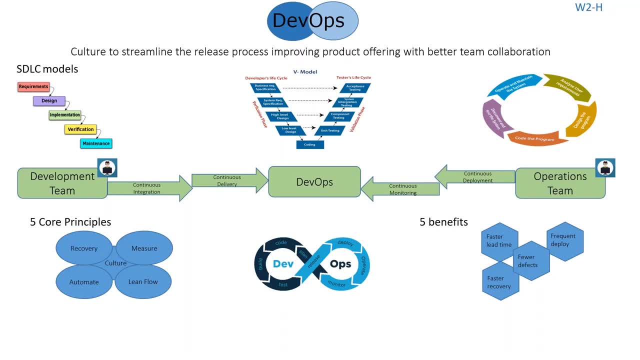 pipeline multiple times and the environment, leading to increase in recovery speed by 24 times through frequent feedbacks. the next one is the footprint: frequent feedbacks through feedback. frequent feedbacks, the process at each and every stage of the development cycle. it makes us easy to estimate, or it makes us easy to. 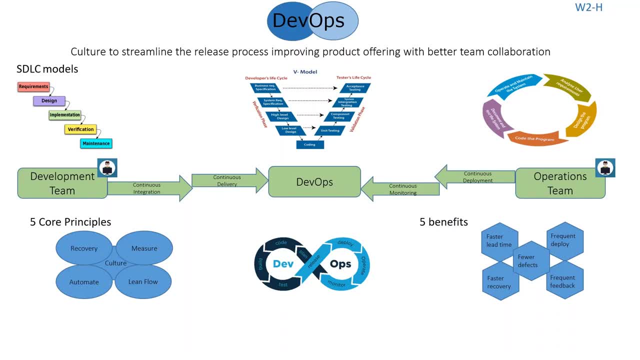 detect where the error is so we can take the similar steps. okay, now i will show you a simple pipeline. let's see this one. so when you are designing the pipeline, the foremost comes is a source code manager. so what is the source code manager? the source code manager is something. 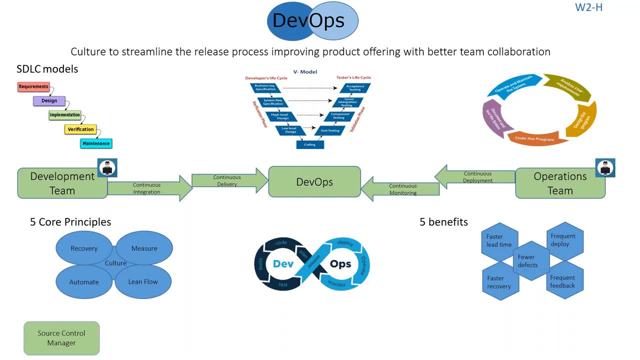 as a centralized server which takes the code and it maintains the versions of the code. it maintains the person who has committed the code, the logs, audit logs, the securities, authentications, authorizations, the connectivity, the backups, so where we can completely have a a source code optimized and maintained over the versions. again, the source code. 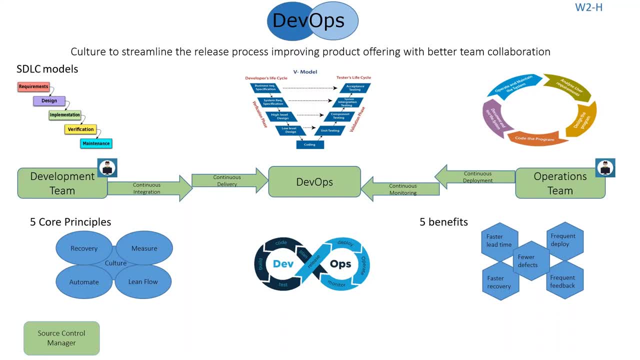 manager provides a lot of other benefits as well, like branching, and multiple developers can work at the same time, the parallelism of progress and, of course, the backup of the code. and next follows the unit test. so what is the unit test? usually so, when we have a code in hand, we usually prefer to code. do the code? 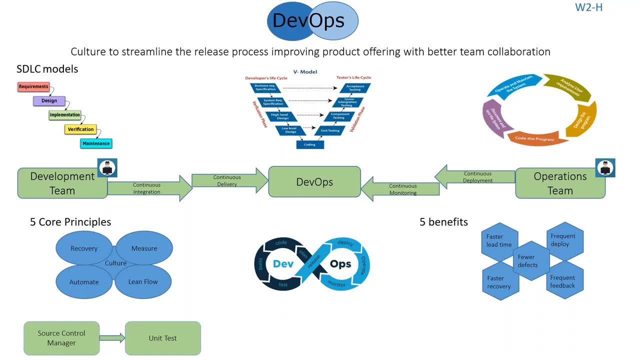 level testing. so that's what we call as a unit testing. so we do entirely a code level testing to check the standards of the code. early, and next comes is the static code analysis, like if my code is exposed to some sort of vulnerabilities, bugs, bugs, warnings or any sims, anything like system details, my database details or my. 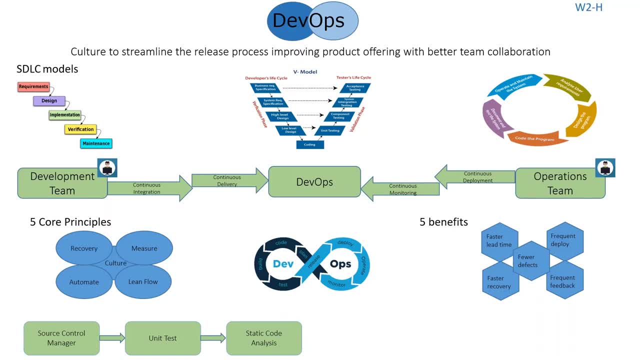 company details or passwords exposed, or the quality of the code to release. so these things will get detected by using the static code analysis tools and next comes the build. this is the essential tool for any releases if we are going to some sort of programming languages. if you take a Java, 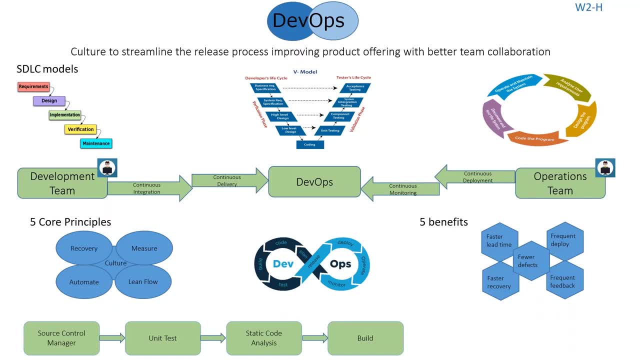 if you take a dotnet, this sort of languages needs a build so that what is build means to package the code so that system can read the code which is ready to deploy. so this sort of packaging is done here on this test and once it is done it is uploaded to the artifact repository and next comes in the deploy. 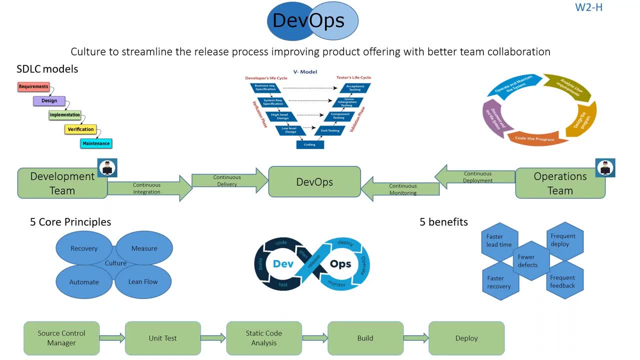 so deploying the code. so why we are using the deployment code in the CI CD pipeline? because we are deploying into multiple servers before going to the production, so the servers can be deployment servers like a delivery at now, develop UAT, SID and production and followed by functional testing. that is the post.